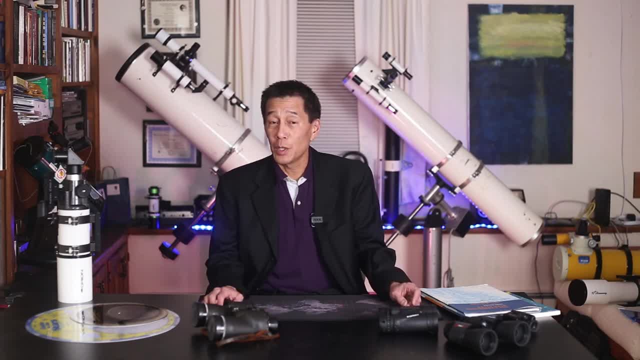 amateur astronomy, and the advice I'm going to be giving you is nothing new to people who have been in this hobby for a while, but if you're coming to this for the very, very first time, I'm going to help you try to avoid certain pitfalls that many beginners make. I'm commonly known as a telescope. 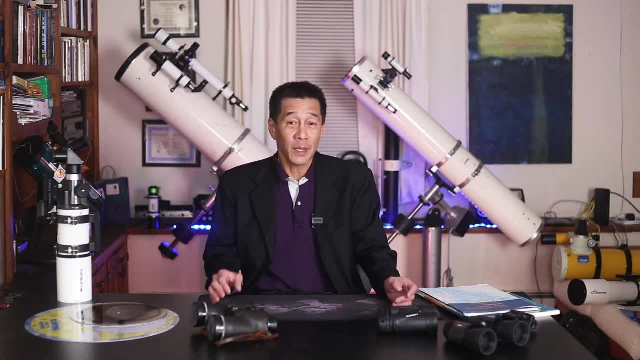 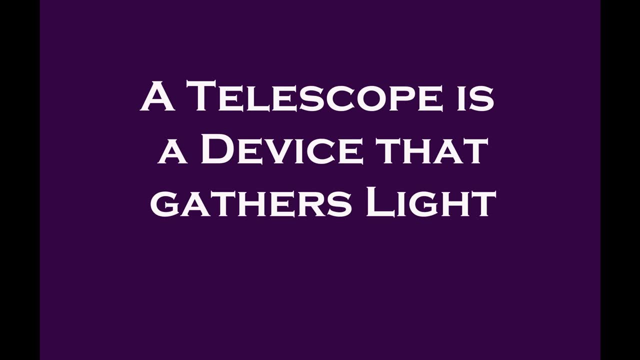 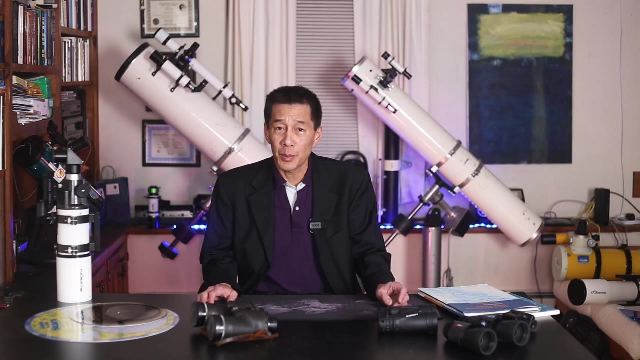 reviewer. so let's go ahead and just begin right there. What is a telescope? Well, first and foremost, a telescope is a device that gathers light. That's its primary function. Many people who aren't in this hobby assume that a telescope's main function is something else. Namely, they think 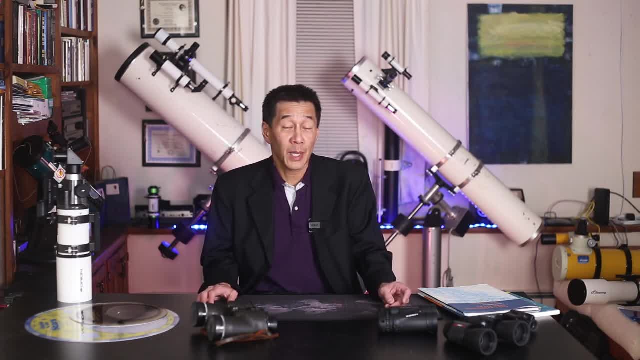 a telescope's main function is to magnify objects, And yes, they do do that. but the magnification is just a mathematical subfunction of the fact that the telescope gathers light. Why is this so important? Well, the human eye can only open up to. 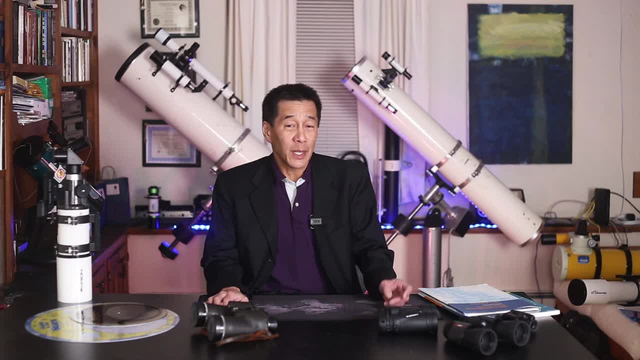 about seven millimeters or so under ideal conditions. so you're only gathering about seven millimeters worth of light. when you step outside, Many of the objects that you see up in the sky are quite large, and the most common example that you often hear about this is the. 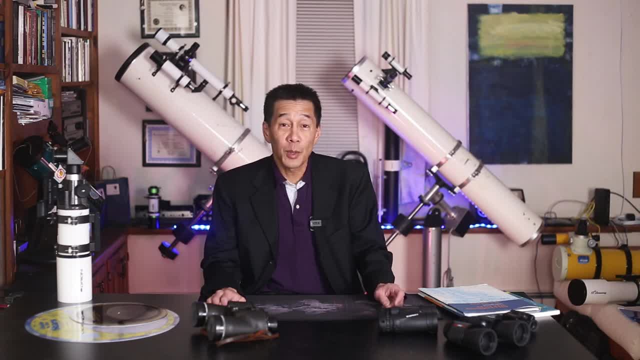 galaxy or M31.. This is visible in the fall and in fact you actually can see this with the naked eye if you're taught where to look. Not terribly exciting to the naked eye, but the actual size of this object is about eight times the diameter of the full moon. It's just hanging up there. 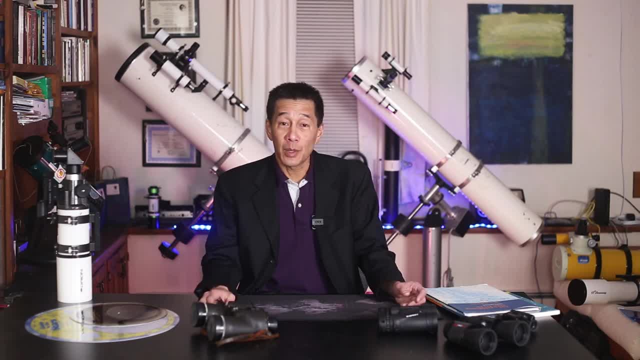 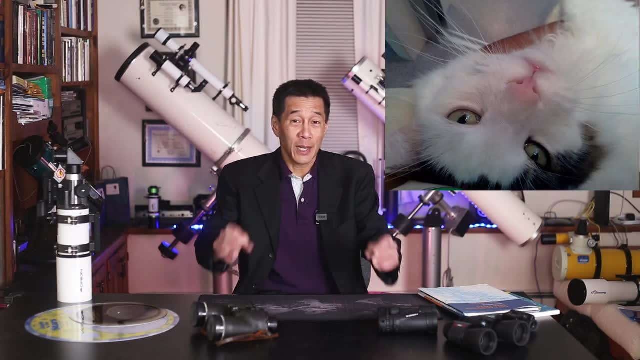 but our eyes will not open wide enough to see the whole thing. I've often wondered what it would be like to be a cat. You know, go outside and have a cat's eyes open so wide that you can't see the much wider. They could really do some astronomy there. Anyway, I've taken these two pictures of 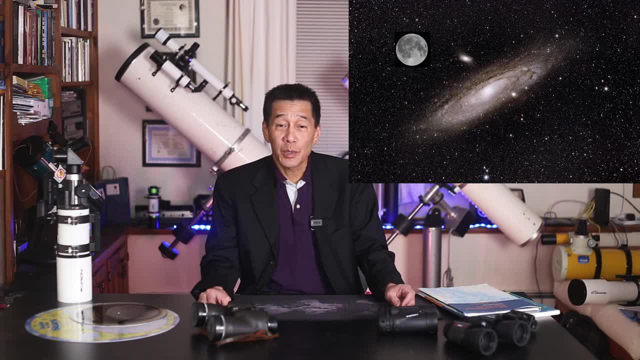 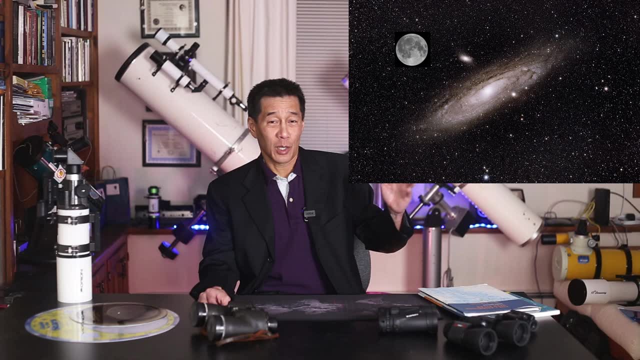 mine of the moon and of the Andromeda galaxy, just to show you how big that object is. No, you're never actually going to see it this way. The moon doesn't get that close to Andromeda and even through a telescope you don't actually see all of that detail. That's a long exposure photograph. 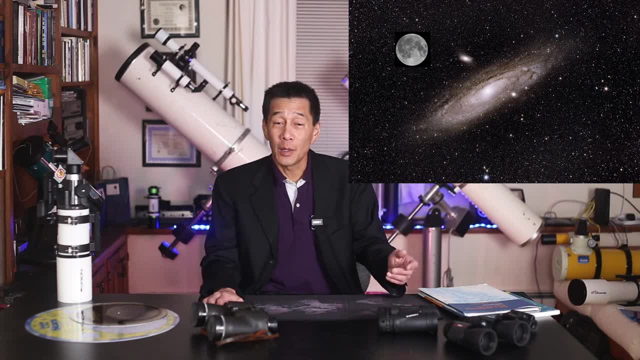 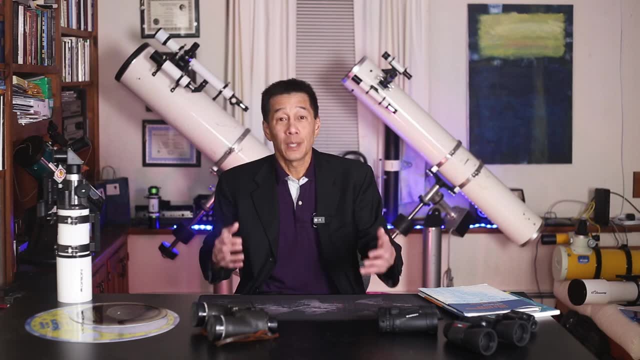 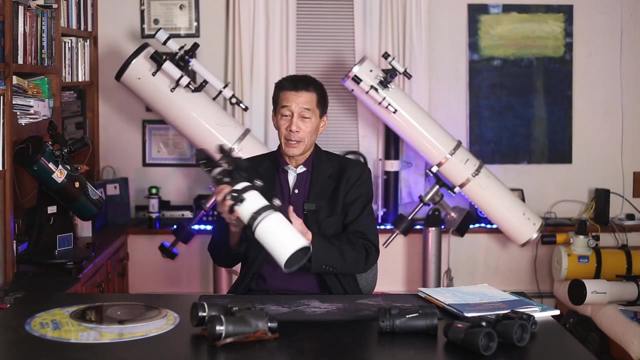 but just as an example of size comparison, that is what's up there, In fact, many of the objects that we're looking at right now. they don't get that close to Andromeda, but our eyes won't gather enough light to see them, So let's take a telescope. Here's a typical beginner's telescope. 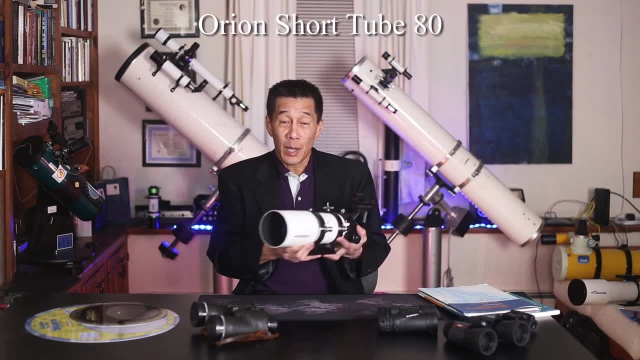 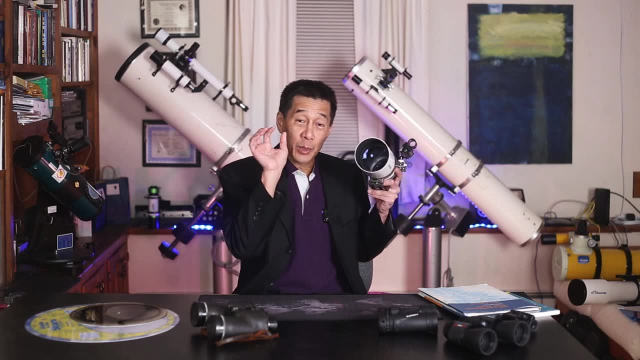 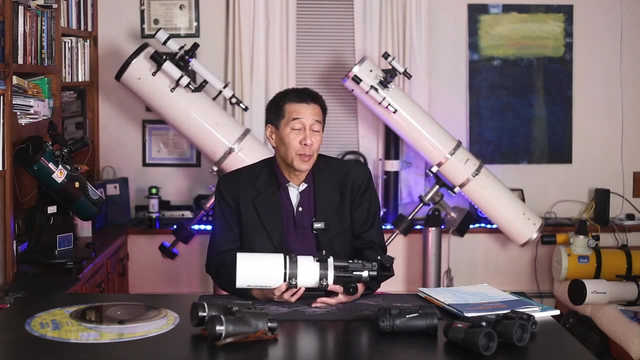 that's commonly recommended. This is an Orion short tube 80.. 80 is the diameter of the telescope, 80 millimeters or about three inches. So you can see, even there, my eye won't get anywhere near the size of this light gathering capability. And this is a relatively small telescope. So even a 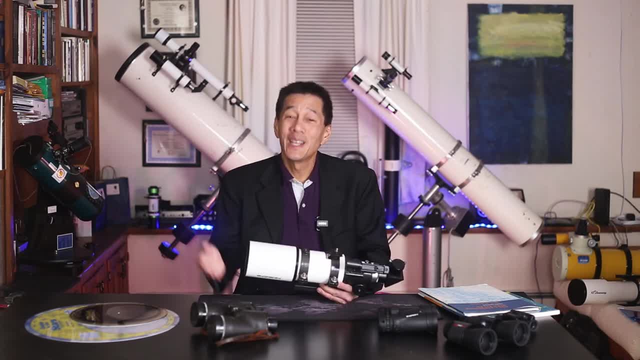 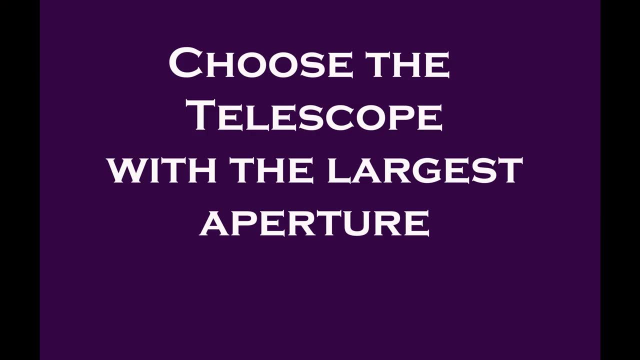 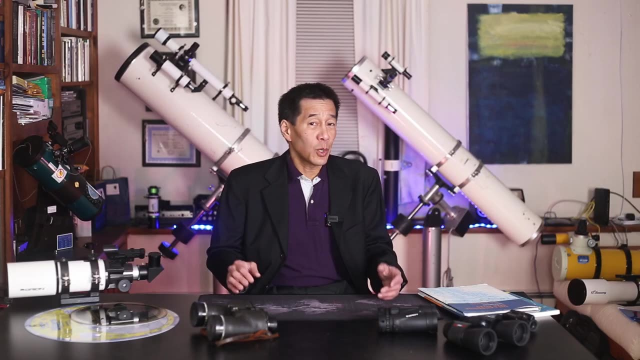 telescope will show you more because it will- yes, you guessed it- gather more light. So here we come to our first important point about telescopes. All other things being equal, choose the telescope with the largest aperture. Now you may ask yourself: why do I need a telescope at all? Why? 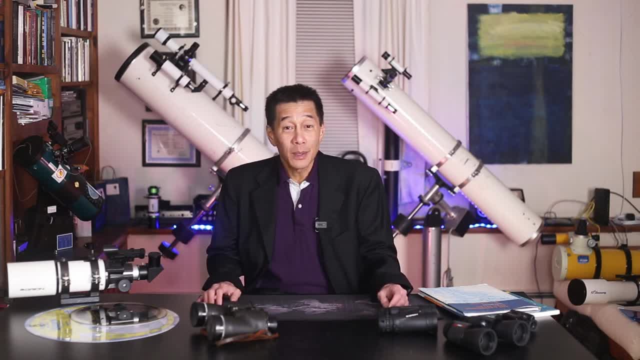 can't I just go outside and look up at the night sky? Well, yes, you can. You can do that. In fact, I encourage you to do that If it's dark out and it's clear right now and you're watching. 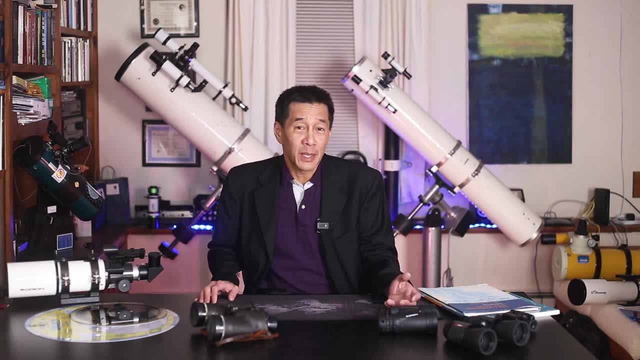 this video, you're going to be able to see the telescope. You're going to be able to see the telescope. Just go outside and look Now. you may say to me: well, I don't know what I'm looking at. 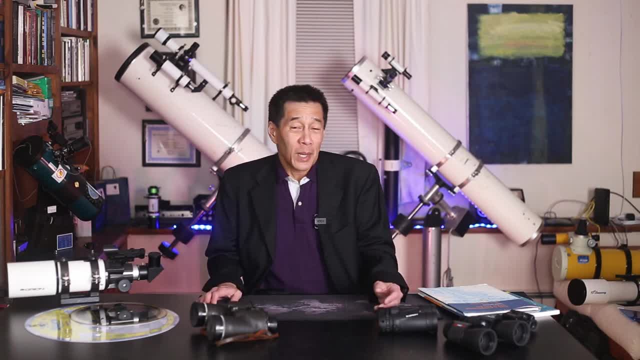 to which I say, so what? You don't have to know what you're looking at to appreciate the beauty of the night sky. Just go outside and admire what's going on around you. Now, if you want to take the next step, what you can do is get yourself something that will show you what's. 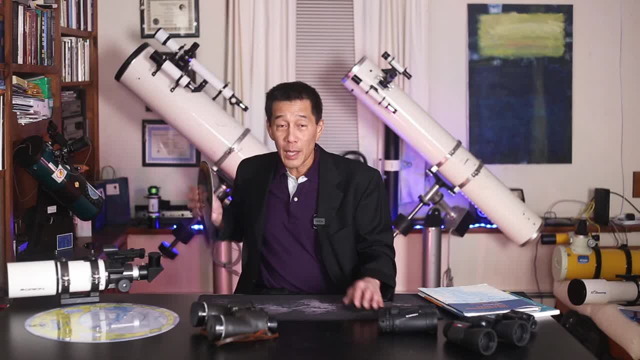 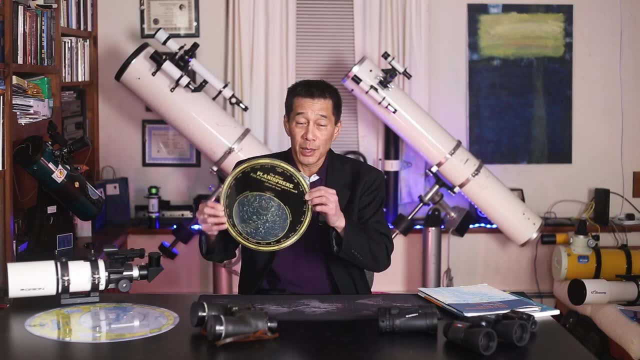 up in the night sky, For example, you can get something called a planisphere. Now, there are many of these out in the market and they're all pretty good, But if you're looking for a pretty good, you can recognize them, because there are these circles here A little bit hard to see. 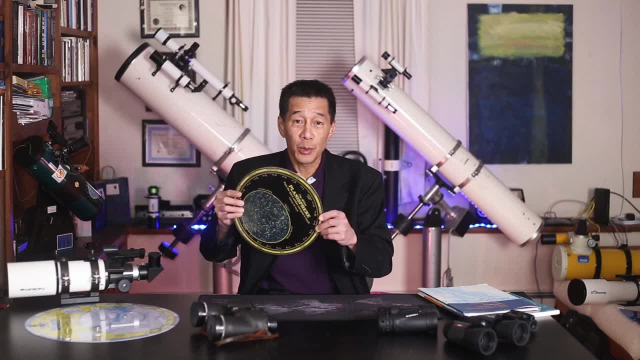 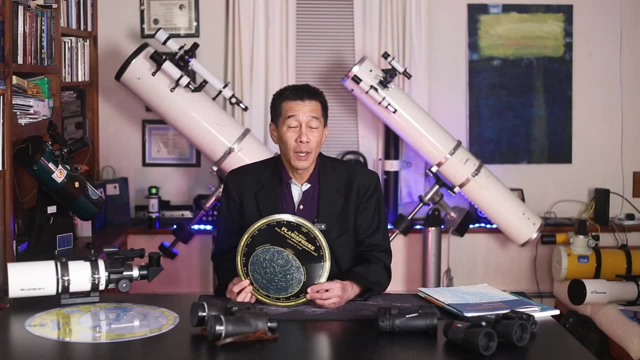 but there are dates and times around the outside and all you do is dial in the correct time and date. You hold this up over your head and it will show you what's up in the night sky. If you do go out, try going out a few hours later and do this again. You may be surprised how much. 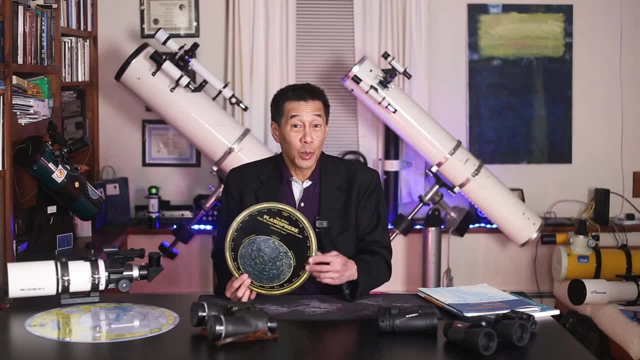 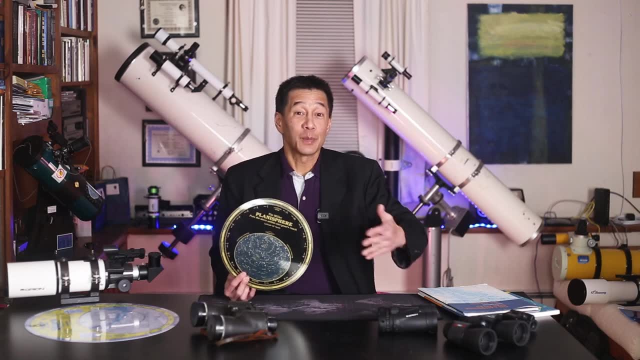 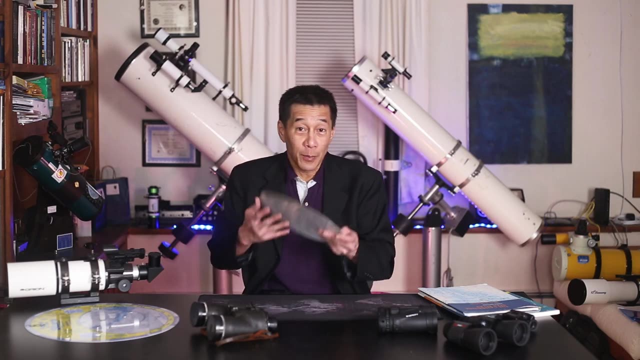 the sky has moved in only a couple of hours. The Earth spins on its axis once every 24 hours, so every hour or so a new 15 degrees of stuff comes up and another 15 degrees worth of stuff sets in the west. You know, back when I was growing up we didn't have a lot of money, so buying a telescope. 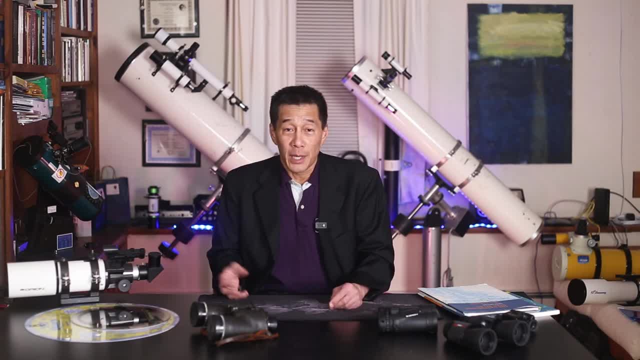 was out of the question And all I did was I went to a library and I got a book that showed the star charts and I sat outside and I looked up. The Earth takes a year to go around the sun, so it 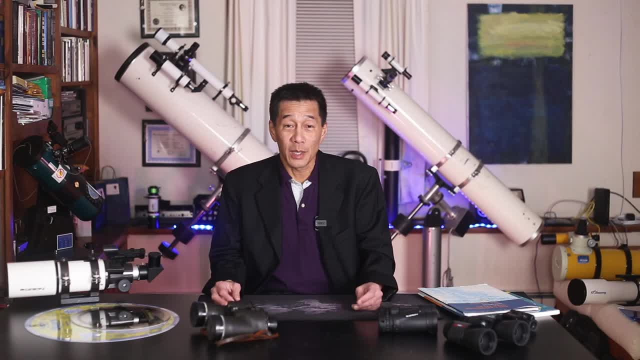 actually took about a year for me to learn all of the constellations and what's up in the night sky, and I never ran out of things to do. I never ran out of things to do. I never ran out of things to do. 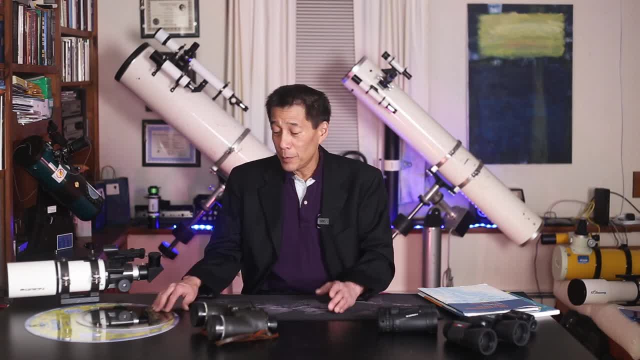 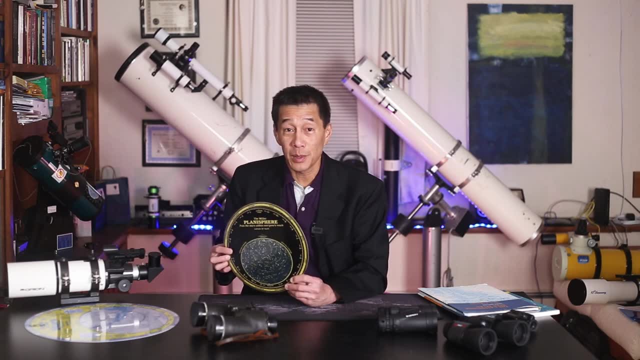 things to look at. You can do much the same thing Now if you get to the point where you learn everything that's on the planisphere. this thing doesn't go very deep. It only shows you the brightest objects in the sky. You can take the next step and get something called. 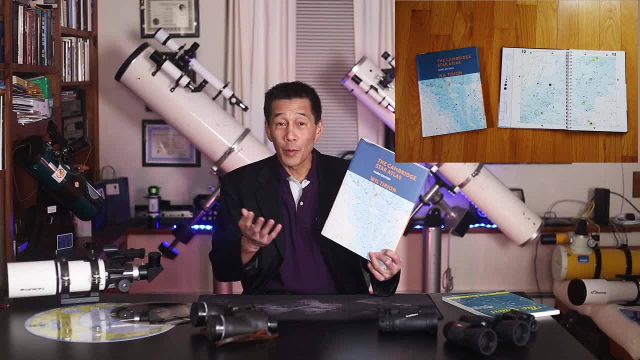 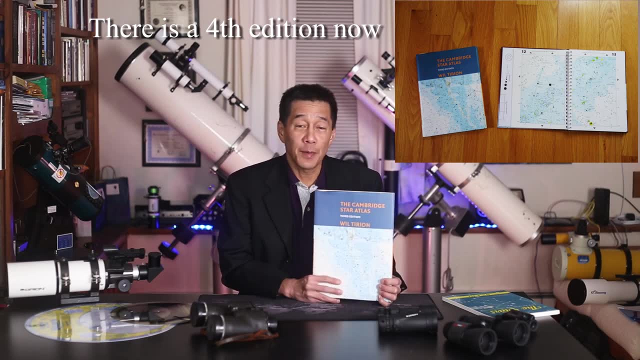 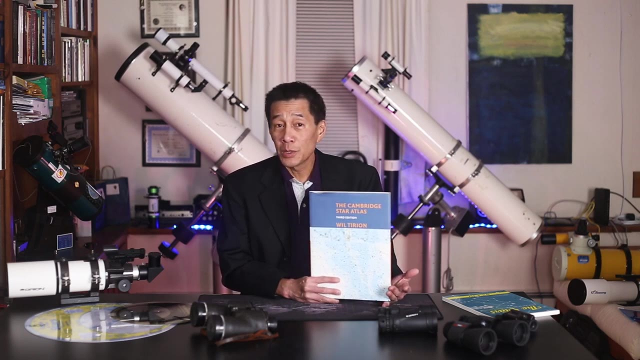 a star atlas. You can get one of these. They're all very good. I have rarely seen a bad one of these. Some of these like this one. the Cambridge Star Atlas is my favorite of the mid-sized atlases. It goes down to what they call magnitude 6.5, which is approximately. 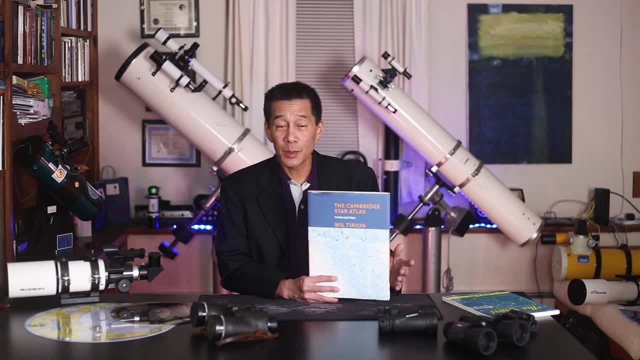 how far the naked eye will go. It is beautifully illustrated and even if you don't know anything about the night sky, sometimes it's fun to just look through this thing and see the different colored objects and just admire what's up there. So let's say you want to know more about astronomy. 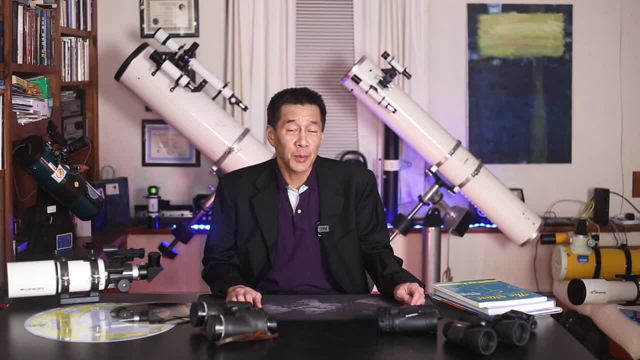 Well, you can get yourself a book, and there are several excellent ones out there. In fact, I have a separate video showing the best beginner's books for you, But I'll just highlight one of them here. This is H A Ray's The Stars. Those of you who know 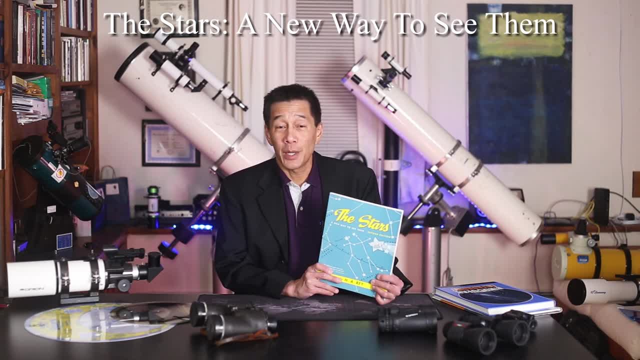 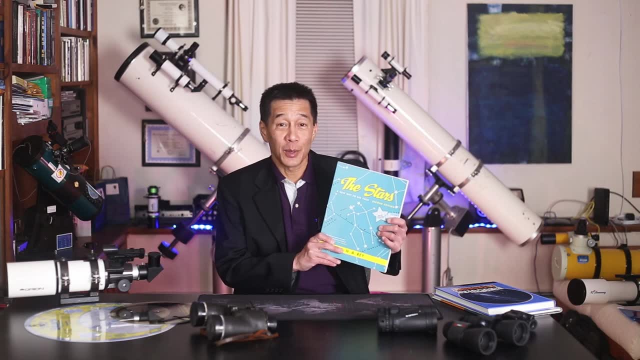 your children's literature will recognize H A Ray as the creator of the Curious George series And in fact, as you look through here, you will immediately recognize the writing style and the drawing style. This is a very non-threatening book for you to get started with and kids of. 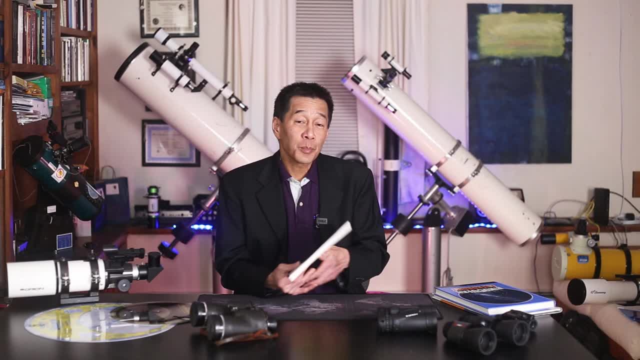 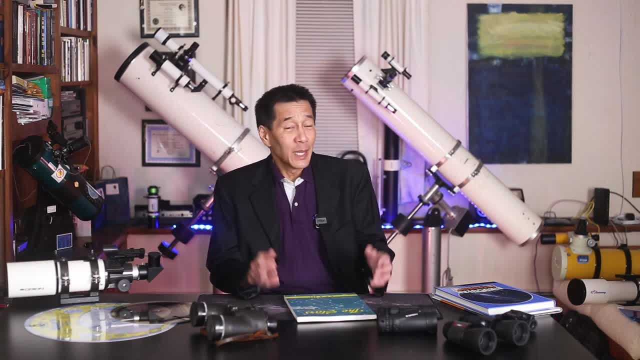 with my star chart and learning the pictures of the night sky. I was about 10 years old and I was looking up and my imagination, I would draw pictures in the sky And the pictures were very much things that a young boy would envision. It's the cowboy, It's the warship, It's the 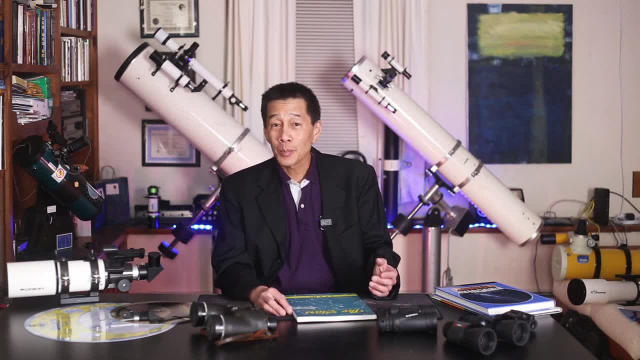 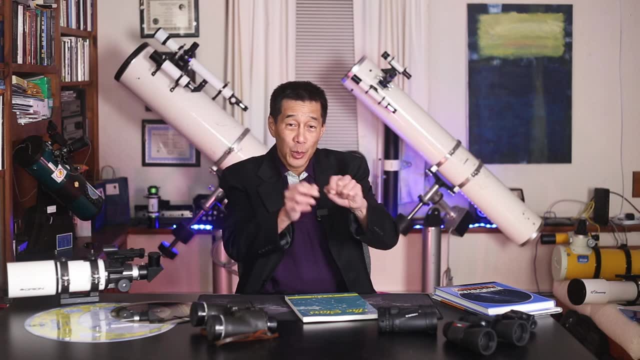 spaceship, It's the firetruck, It's the astronaut, And I got to the point where I really loved my pictures in the sky And I got out my piece of paper and I drew them And one day I brought them in to my teacher and I was like I'm going to get this book And I was like I'm going to get. 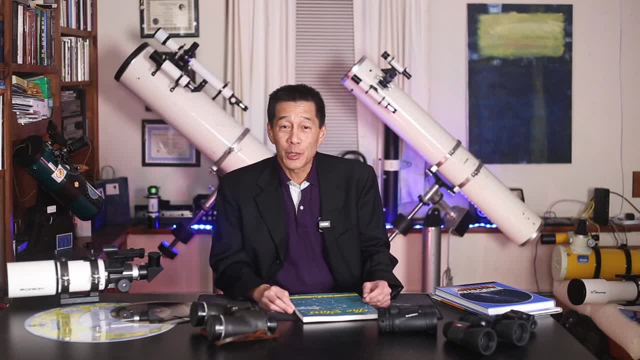 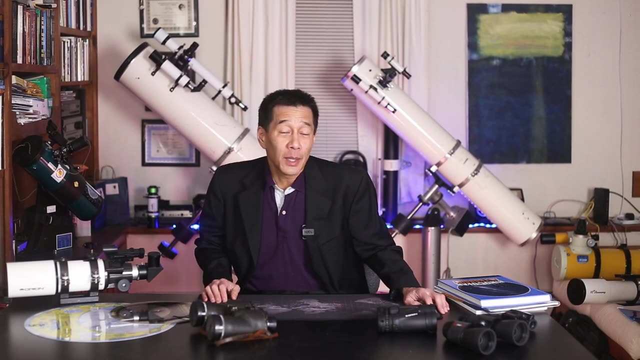 had visions of fame and fortune in my head, and the teacher just deflated me. It turned out that the constellations have all been established a long time ago and the book that deflated me that day was HA Ray's The Stars. Now, let's say you find the purchase of a telescope too daunting, or? 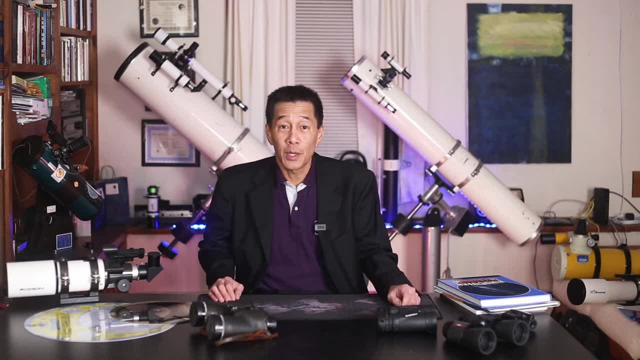 too expensive at this point. That's fine, also because what you can do is get yourself a pair of binoculars just like these. I've got a few of these lying around Now. binoculars are actually a great introduction to astronomy, and they're actually better than buying a cheap telescope. 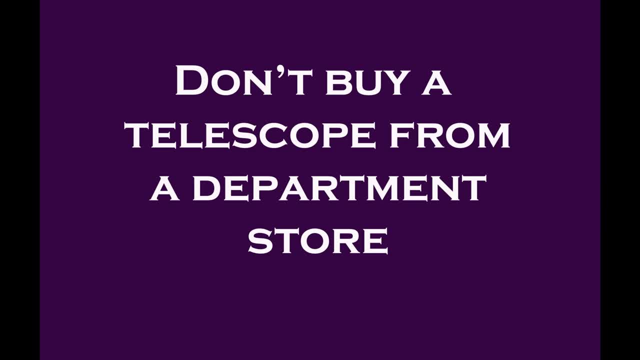 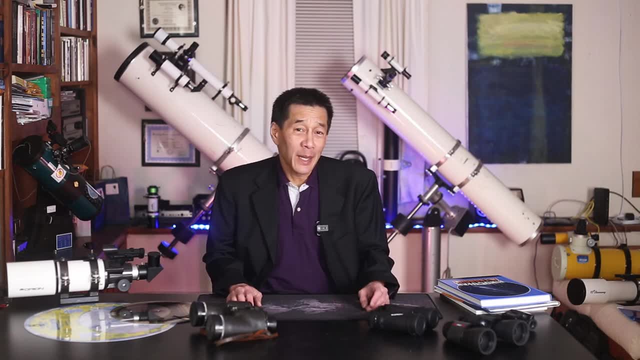 Please do not buy a telescope in a department store. I'll go through this a little later on, but those things are hobby killers. They are the bane of our industry, and it may seem counterintuitive, but you're actually better off not buying a telescope at all than getting one. 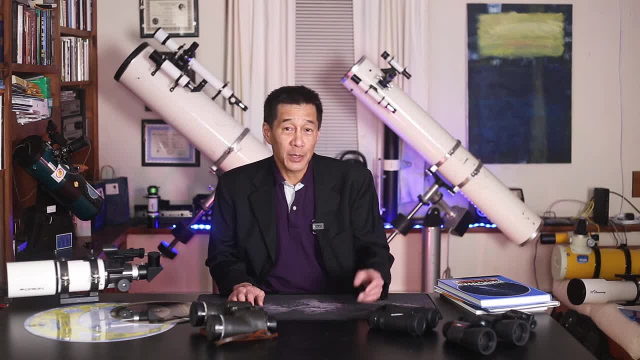 from a department store, But very often in that time you're not buying a telescope at all. that same place you'll find binoculars for sale that are okay. I don't understand why this is so. Binoculars are kind of a complicated optical instrument, but cheap binoculars are almost 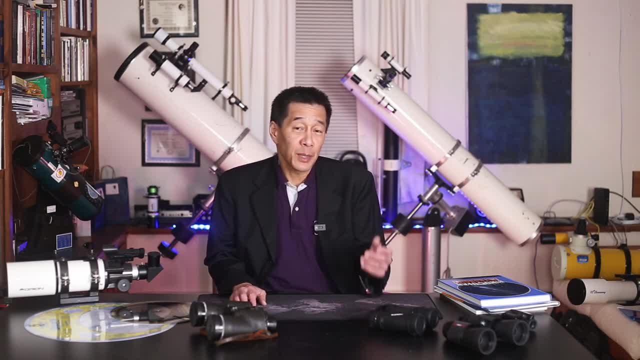 always better than a cheap telescope. Now, binoculars are rated by two numbers. You'll see one number, an X, and then another number. You'll see 7X35.. You'll see 7X50.. You'll see all sorts. 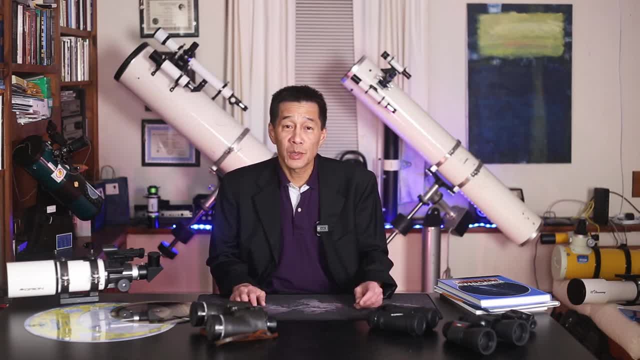 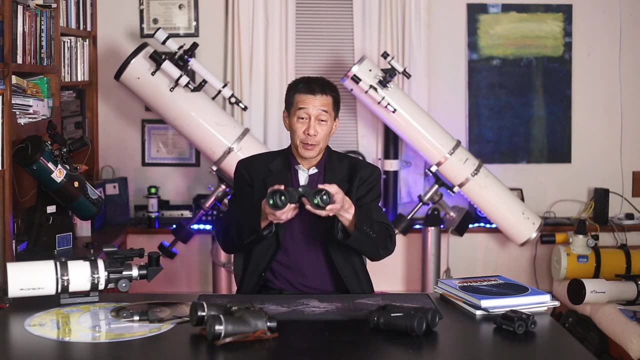 of numbers. The first number is the magnification and the second number is the aperture in millimeters. Based upon what we've discussed before, you know what you want. You want the binoculars that have the most aperture. I've got a couple of these here. These are 7X50s, 7 magnification. 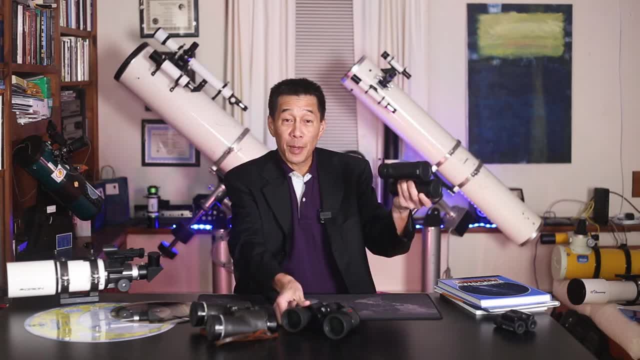 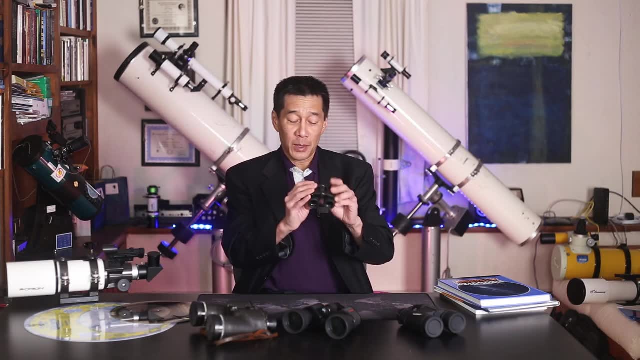 and 50 millimeter aperture. These are 8X42s. 42 millimeter aperture, 8 power. These little ones here are 8X20.. The guys at the astronomy club sometimes make fun of me because I use these things. 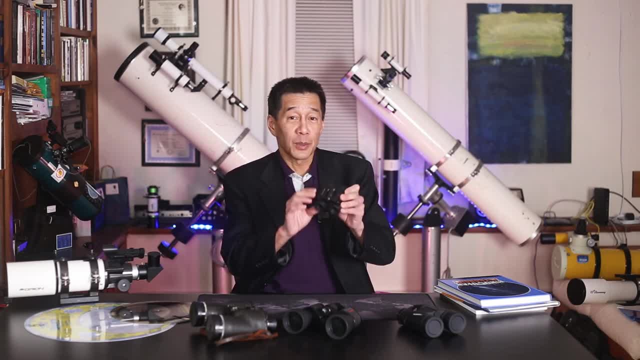 But still they still gather 21 millimeters worth of light, which is far more than the 7 millimeters that your human eye can see, And you might be surprised just how much you can see even with a bad pair of binoculars. Now, many of us have a pair of binoculars lying around somewhere in the house. 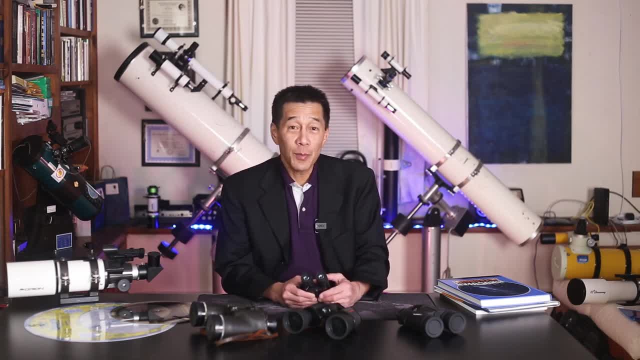 Maybe they're gathering dust in the shelf somewhere. If you have one of those, take them down off the shelf. You can put them outside on any clear night and just point them up at the night sky and start sweeping around. I think you might be pleasantly surprised just how nice the views are. 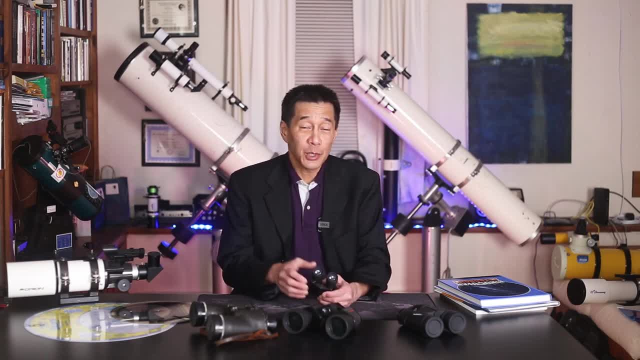 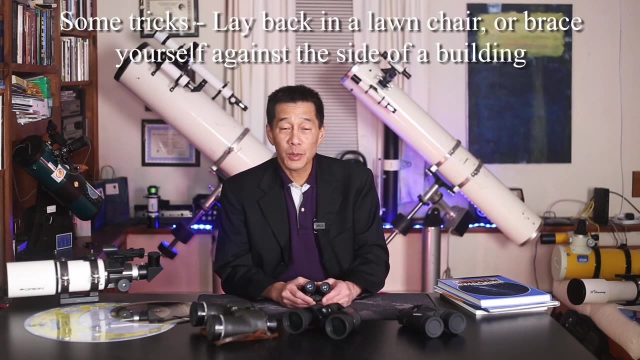 So now we know that you want the highest possible aperture, but, somewhat counterintuitively, you want the lowest possible magnification. The limiting factor to how much you can see isn't the magnification, It's your ability to hold the binoculars still Above about 7 power. 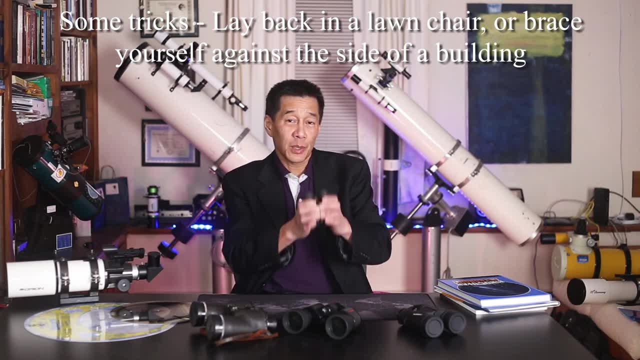 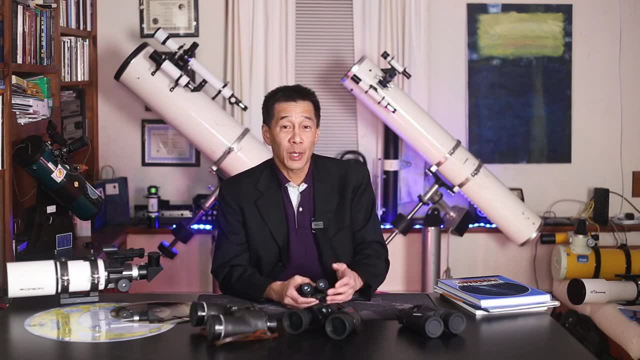